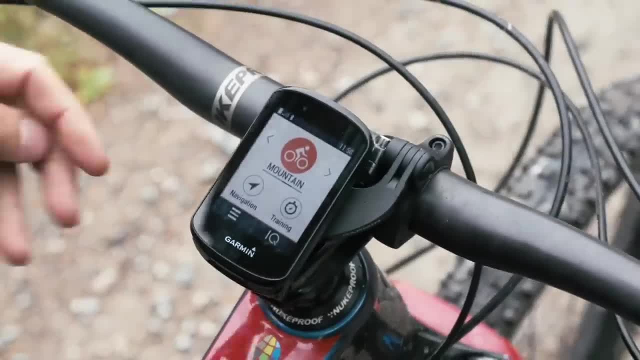 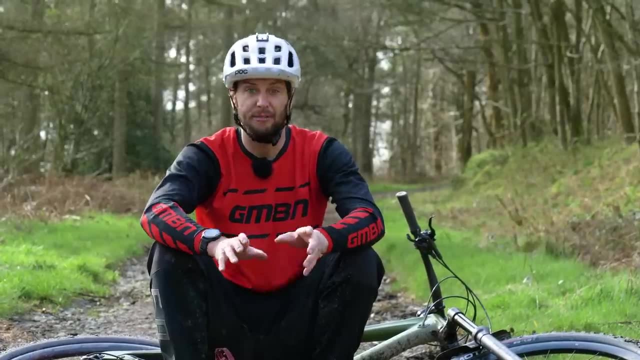 way. Another little thing that can help mentally is that if you have a cycle computer on the front of your bike, you can see the stats and see what you're pushing out, be that heart rate, speed, average speed. obviously All these things in your mind can help you pace yourself. 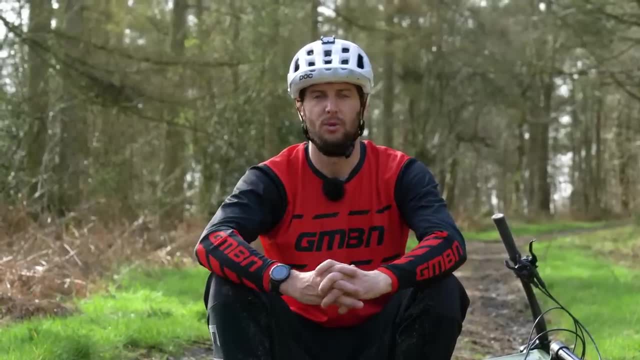 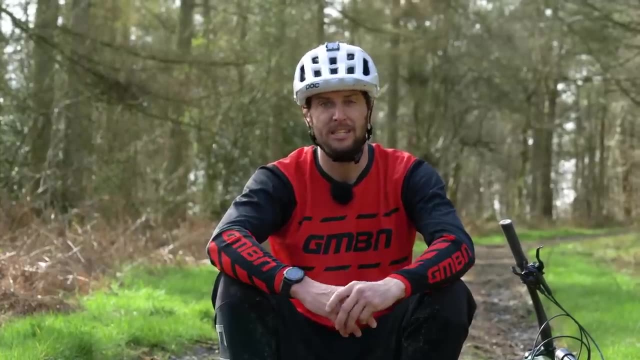 and help you get to the top that little bit easier. All of these little, small wins can really add up to affecting you mentally and giving you a real positive boost. Another great little tip actually is, if you're riding with friends, that can help take your mind off of it no end. 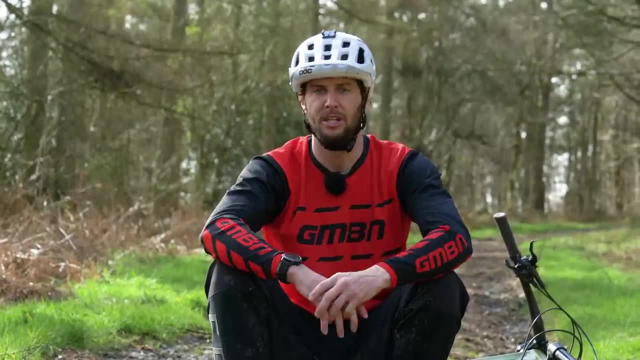 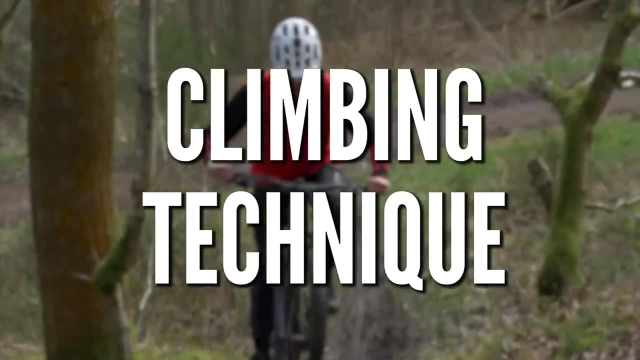 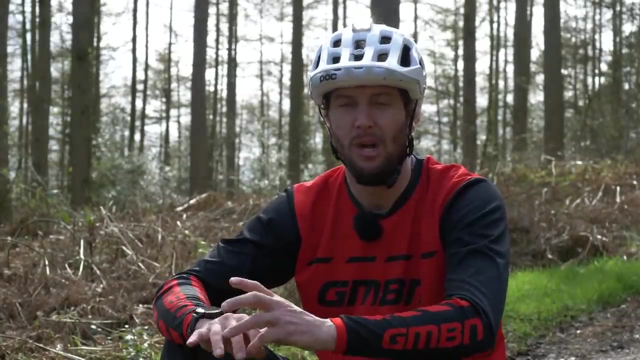 and the time will fly by. Now. we've talked about the mental approach. I think we should start tackling some actual climbs Now, when you're tackling that uphill nemesis of yours, having the correct technique and body position is going to be crucial. We're going to take a look. 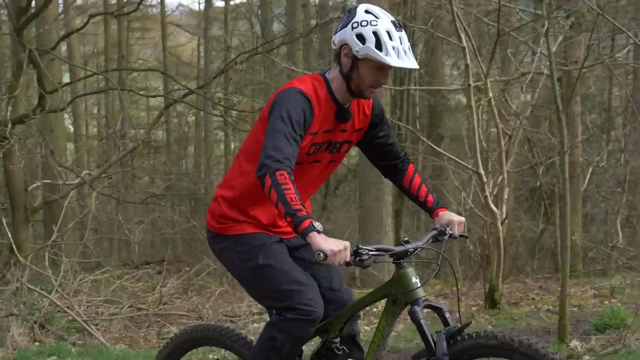 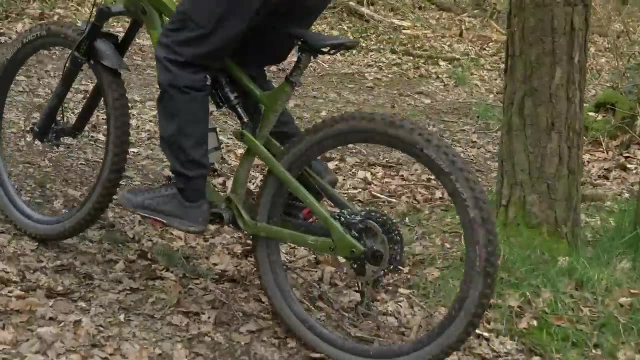 here at what a good basic position is and what you should be doing and when. Firstly, when climbing, you'll want to stay seated the majority of the time, unless the climb it takes. you need to stand up, such as it gets really steep or rough. This will help keep your 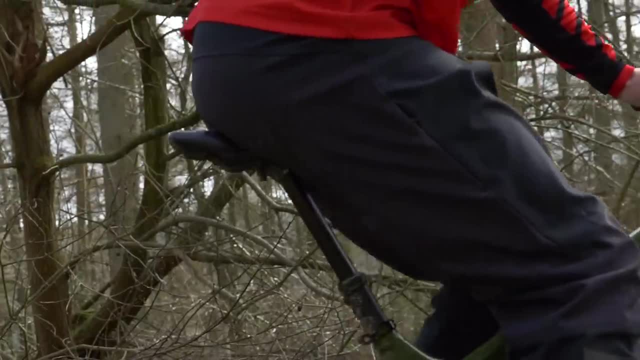 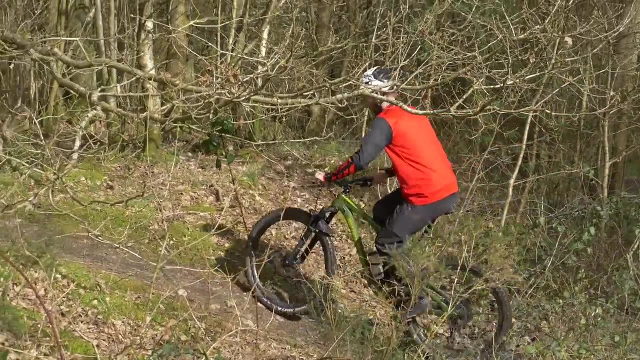 weight back over the rear wheel to stop it slipping and give you much needed traction. You'll want to assume a fairly neutral riding position. However, if the gradient of climb changes, you may find yourself shifting your body weight forwards or backwards for grip. 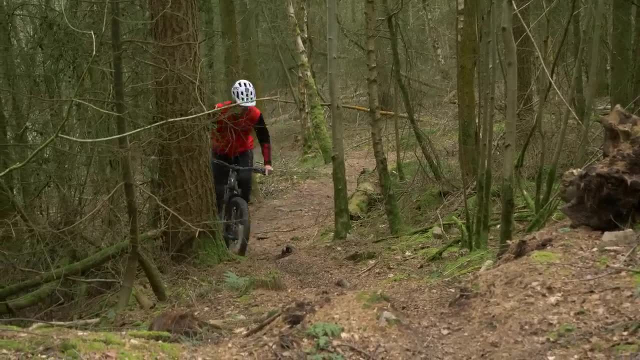 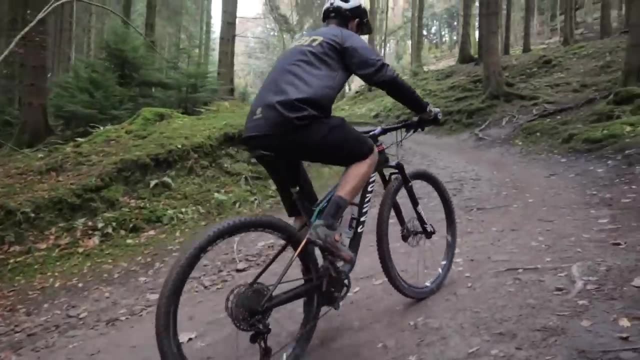 While seated, you'll also want to keep your upper body lent forward to stop the front end going too light and picking it up, making you go wobbly and lose control of steering Arms bent to absorb any impacts and to move the bike around. 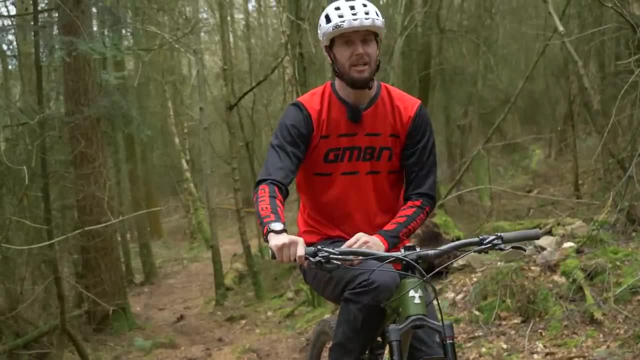 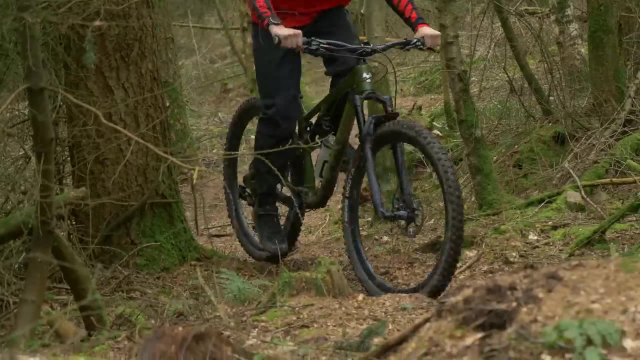 Now gearing. Let's talk gearing for climbing, because it is a really important one, and it can make all the difference whether you actually make it up or not When you're hitting these short, sharp little climbs like this, being in the correct gear, 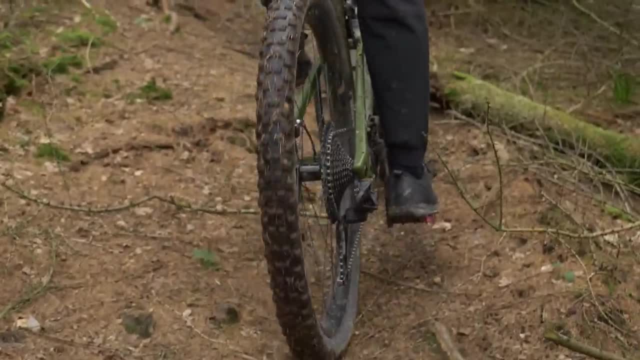 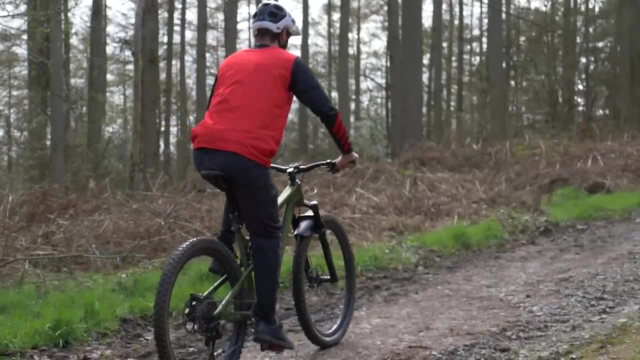 beforehand is hugely important, as it's very difficult to change when the pedals are under such pressure. Having said that, when we tackle these longer, more mellow climbs, finding a right gear for the right cadence for you is also just as important, as it means you can just nicely spin and 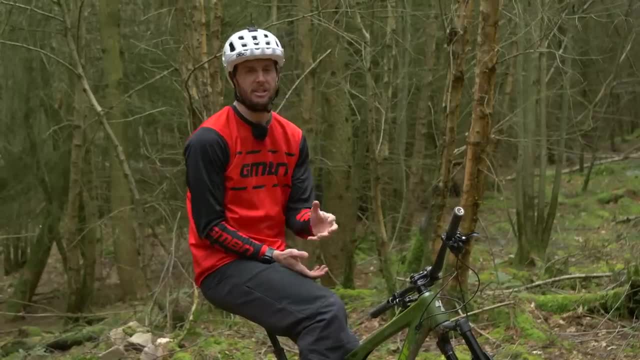 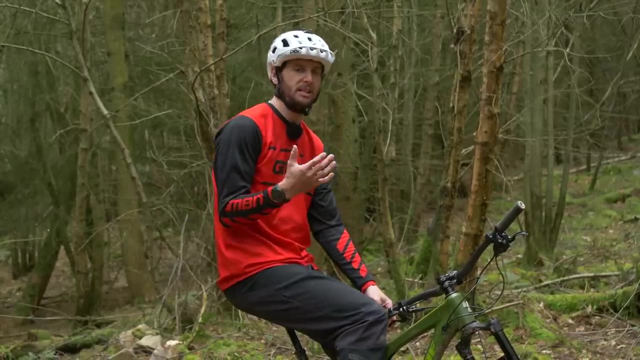 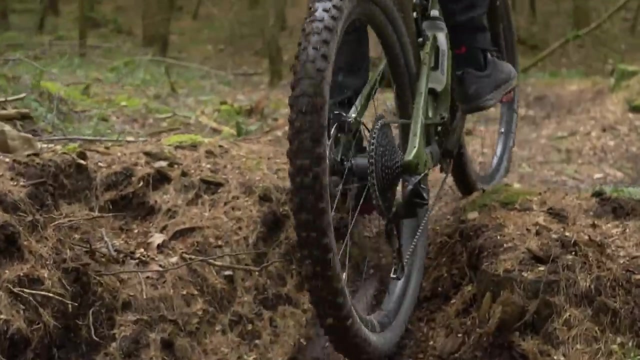 keep a steady pace the whole way. As I mentioned, getting your gearing right before the climb is really important. You want to enter the climb in that gear that you're going to be confident you can get up in. Trying to change gear whilst going up these steep little climbs is going to sound horrible. It's. 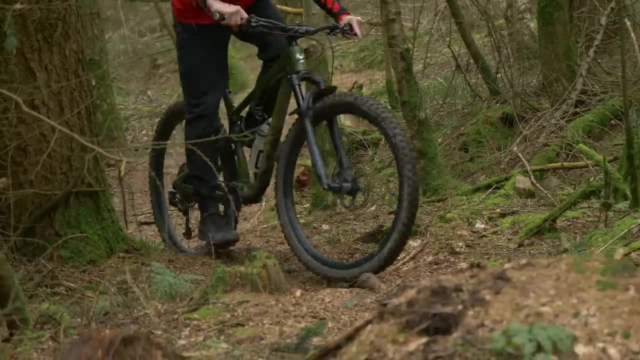 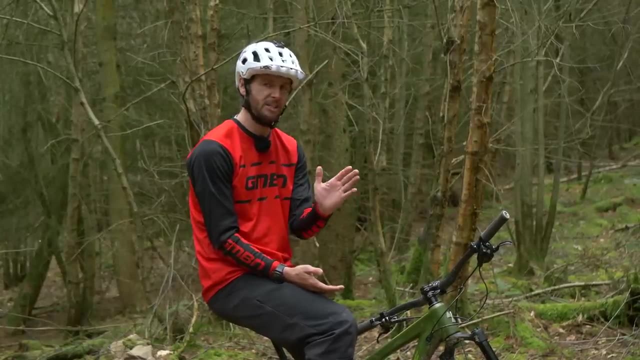 going to sound like you're murdering your mech. Oh, gear change. Come on gears. They didn't like that. You're going to do damage to your drivetrain. It's going to find it very hard to shift through the gears because of the pressure it's under. Again the same with cadence, Once you've. 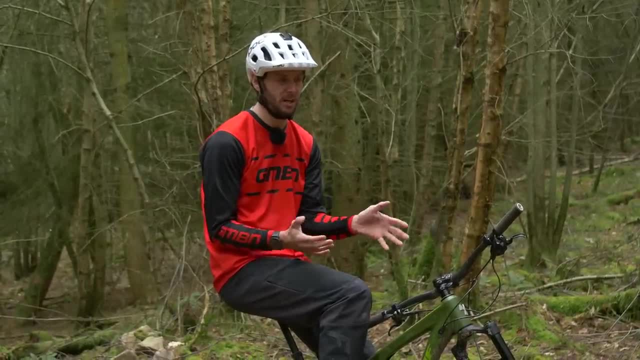 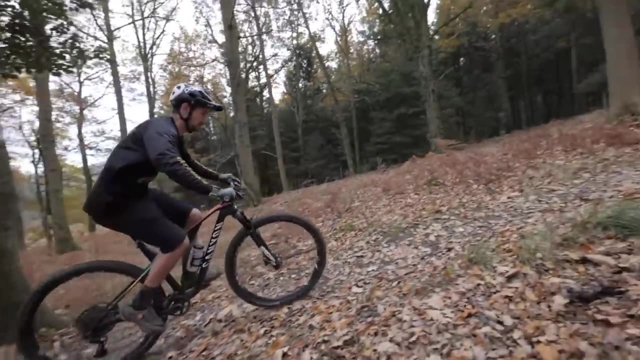 done a few climbs and got used to the gradients and what you're fitness levels are, you'll find out soon what average cadence you'll be able to keep up. Keeping that the whole entirety of the climb will really allow you to get up feeling fresh-ish at the top. 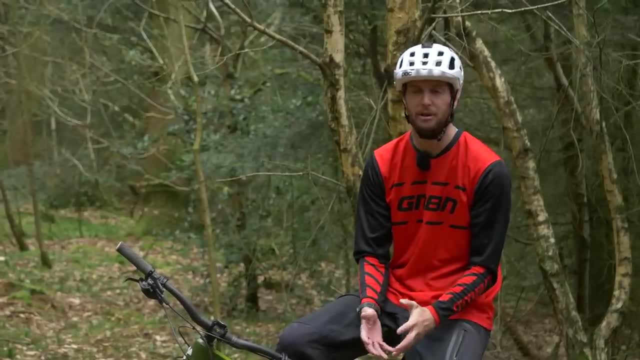 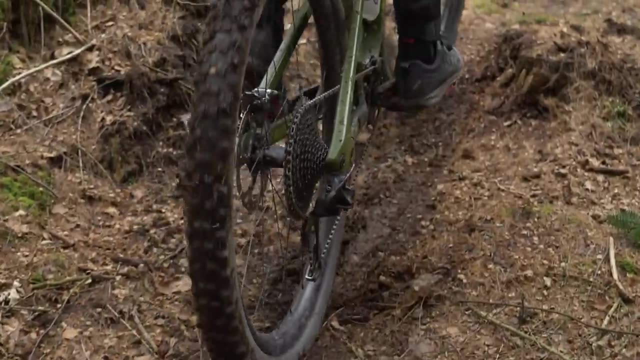 hopefully. Lastly, think of the gearing you've actually got on your bike. Now. most bikes these days come with a one by 12 setup. That big ratio at the rear should be enough to winch yourself up almost any climb. However, if you do live somewhere especially, 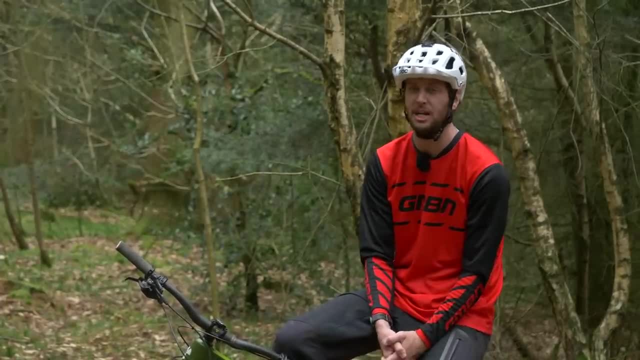 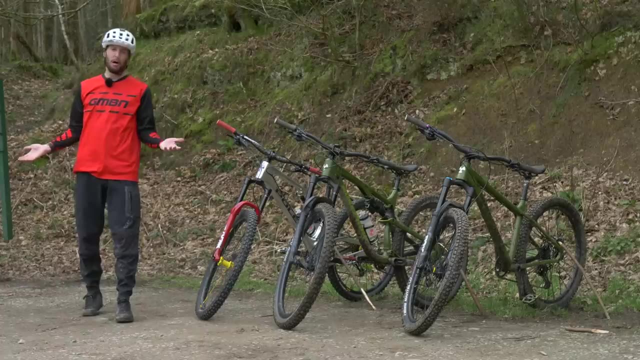 mountainous. I'm a bit jealous, but you might want to think about a smaller chainring on the front to make it even easier. Speaker 1. Bike choice can play a massive role in how easy you find the climbs Wrong bike struggling. 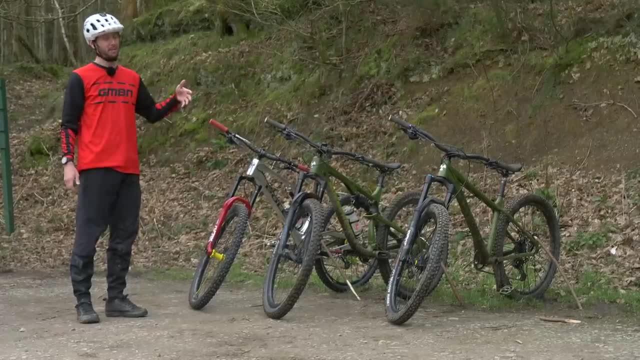 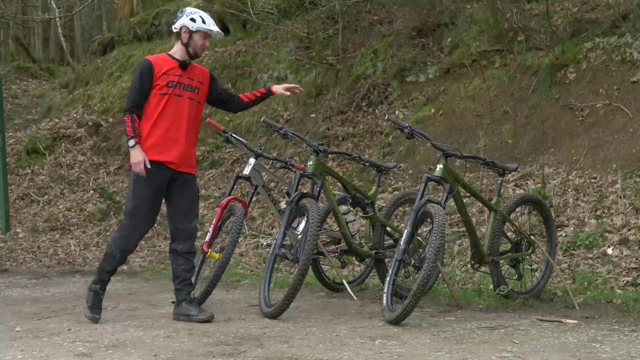 Right bike, perfect. I've got three different bikes here lined up with mine. I've got my Polly Stamina 180.. She'll go up and down but she much prefers the down. We've got a Nukeproof Reactor Trail Bike. This is a 29er, 130 mil. I would say the jack of all trades and does them all. 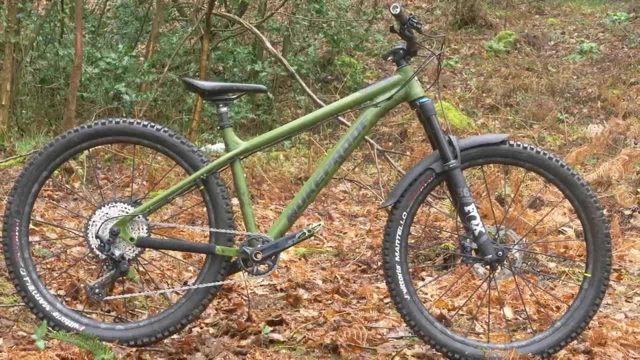 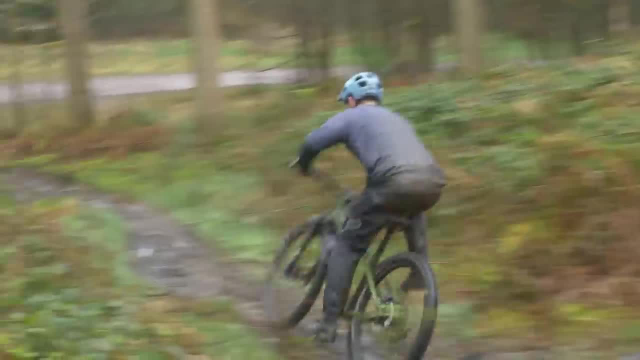 pretty good. Lastly, Nukeproof Scout Speaker 1 A hardtail, The best on the climbs, I would say The most efficient, lightest and easiest, but probably a little bit bumpy on the way back down. All three of these bikes are going to go up. 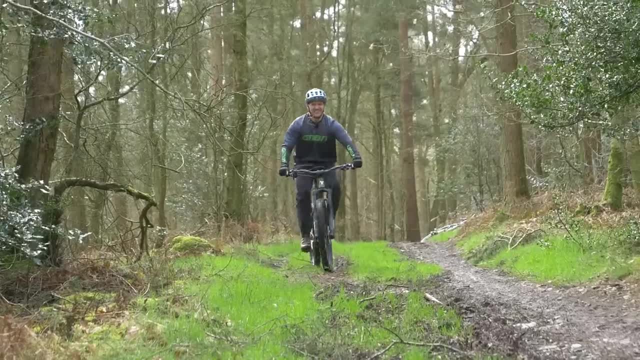 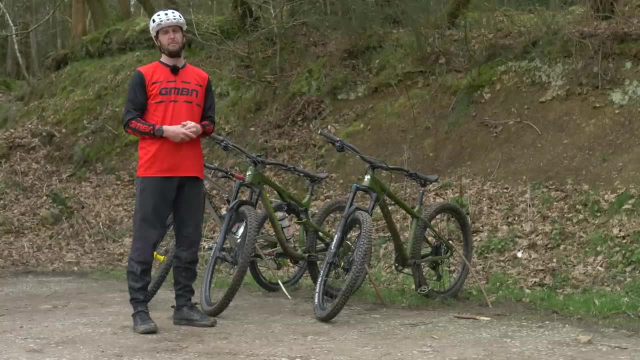 but one of them is far more suited to it than the other. That is the hardtail. When you're thinking of buying your next bike or you're riding- generally tackles, mostly uphills- have a real think about what the best bike for you is going to be. 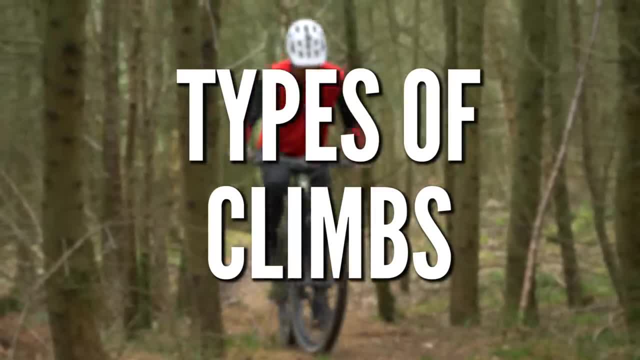 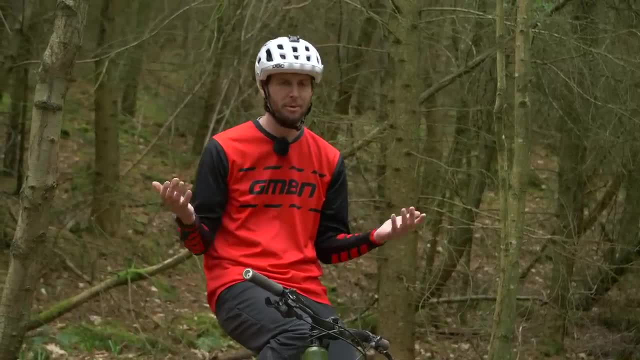 Speaker 1- Bikes. Speaker 1. You've nailed the basics, you've, you've chosen your bike and you've got, hopefully, a bit of fitness. what about the types of climb? We're going to take a brief overview now of what are the types of climbs out there. 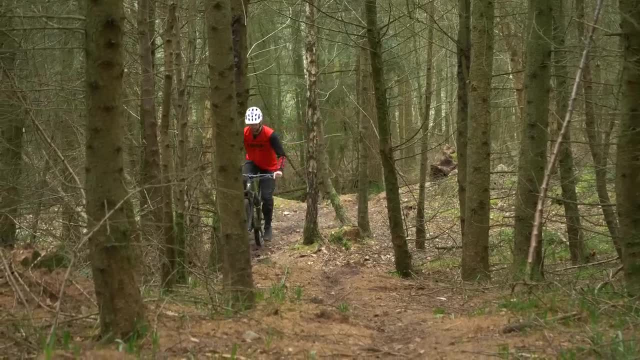 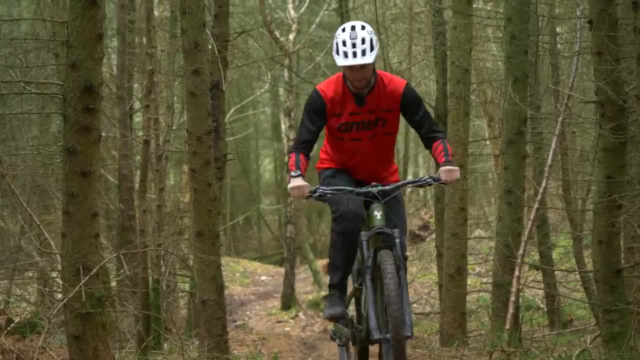 that you're most likely to tackle and how to tackle them. So our first type of climb is the short and steep climb. Now, these are quite tricky. You're going to find yourself with more body weight over the front. You want to try and tackle them with more intensity. 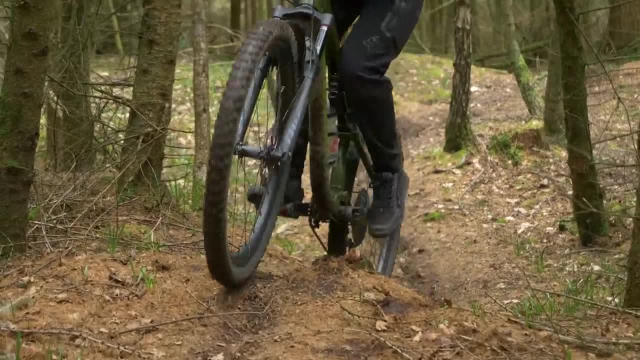 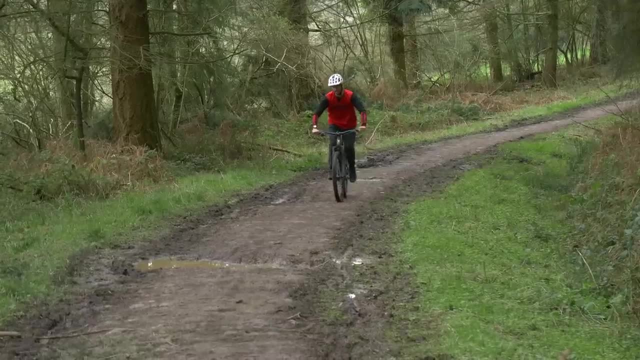 because they're generally shorter as well. On these short and steep climbs, you're also going to want to really drive through the legs, putting the power down for grip and traction. Now, those long and mellow climbs, These are the ones where you want to settle. 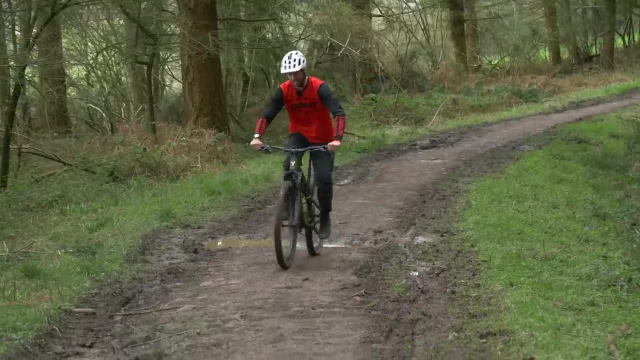 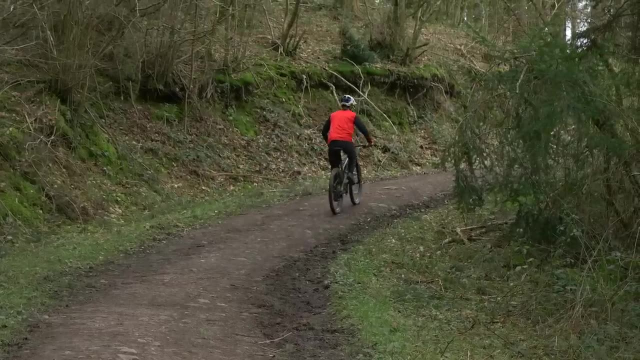 into that rhythm. we spoke about Finding that good cadence and also using a cycle computer, if you have one, to keep an eye on that heart rate and speed to make it all the way to the top. Also, don't be too aggressive on the pedals. 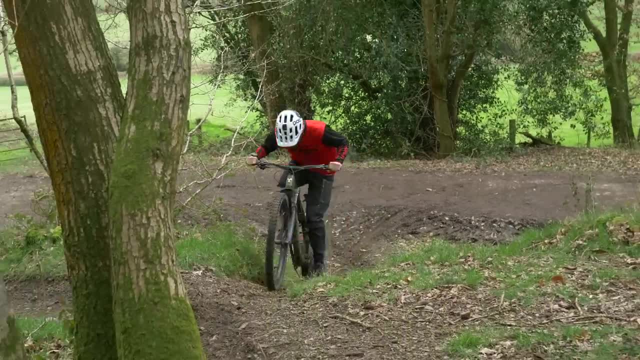 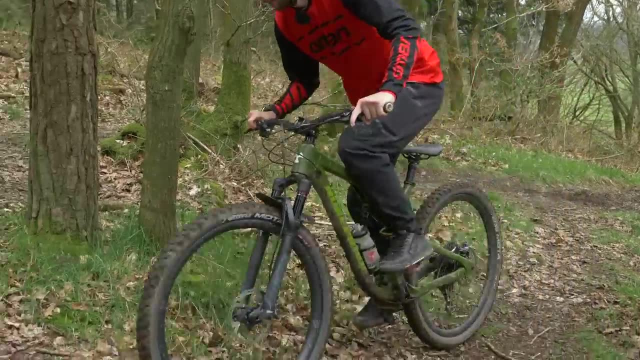 Now the techy climbs. These are the trickiest to master generally and often the hardest to get up. They're going to require more movement on the bike and more thought of gear selection, shifting your body weight and line choice as well. 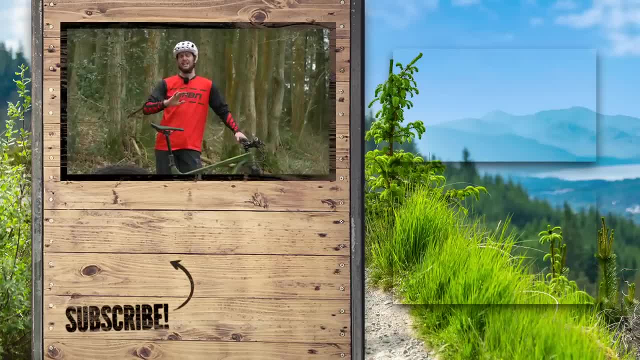 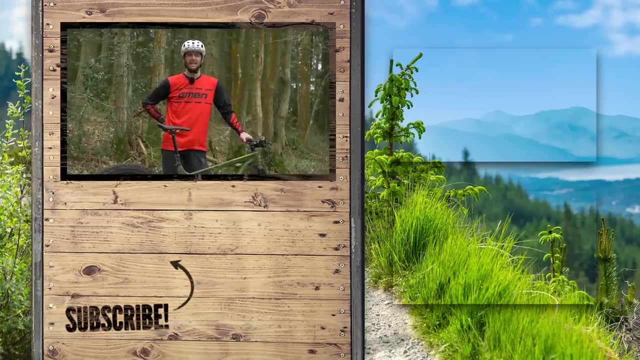 Well, that sure is some meters we've put in today to hopefully help you tackle any climb on your mountain bike. Now, if you want to see a video on climbing mistakes that I made, just click over to the site here. If you want to watch more, don't forget. 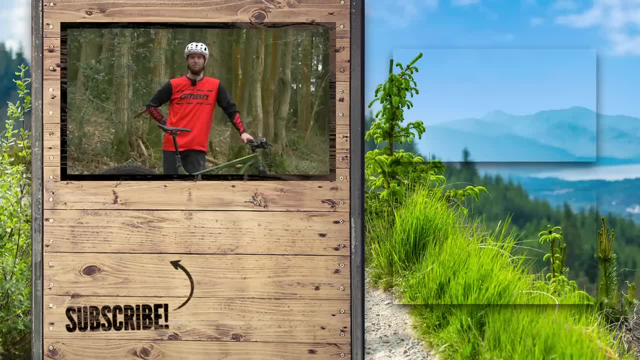 hit subscribe and like us and also follow us on social media. It would be fantastic. 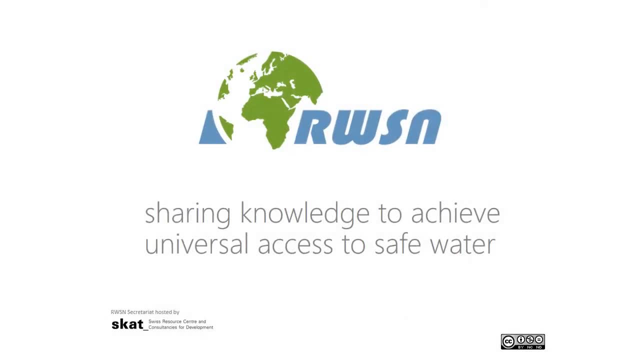 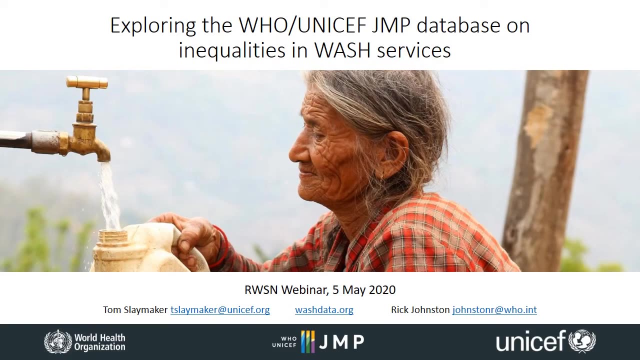 Welcome to the RWSN webinar on exploring the WHO-UNICEF JMP Global Database on Inequalities in WASH Services. The WHO-UNICEF Joint Monitoring Programme, or the JMP, was established in 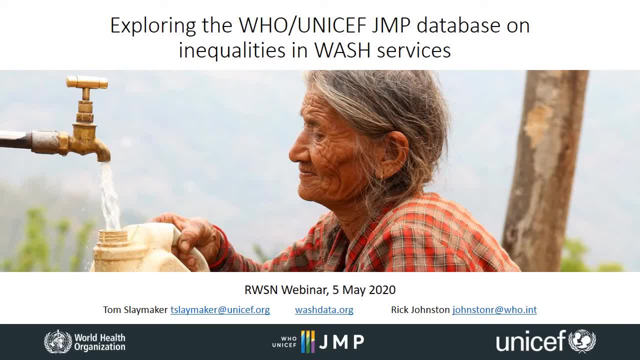 and Rick Johnston, who leads the WHO side of the JMP. 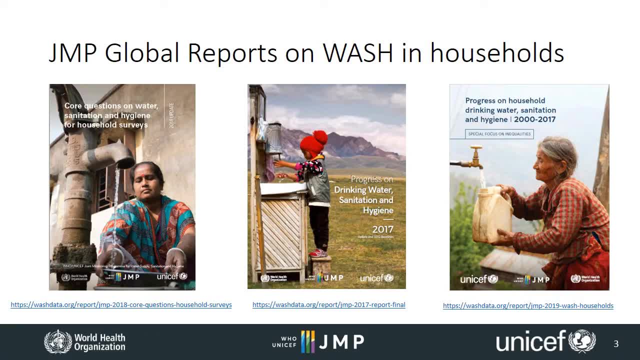 The JMP was previously responsible for monitoring the Millennium Development Goals and is now responsible for global monitoring of the Sustainable Development Goal targets related to WASH.